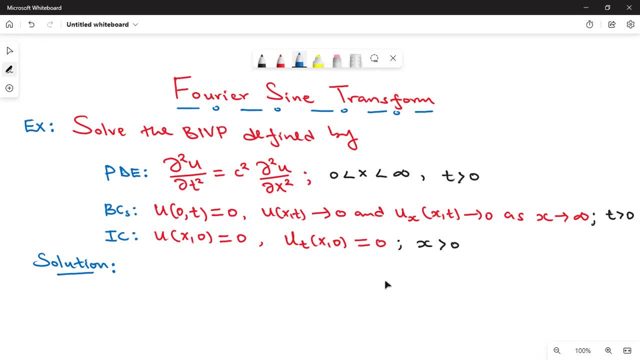 So we need to use Fourier sine transform. But you see, at some point you might not be even told which transform to use. So what we are going to do is we are going to use Fourier sine and Fourier cosine transform. So what will guide you is the boundary condition at the starting point, at the lower end. 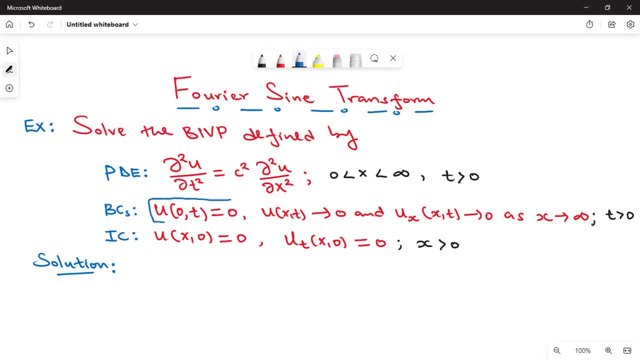 That is what will guide you to know which transform you are supposed to use. If the boundary condition at the lower end, if you know the solution at the lower end, then we use Fourier sine transform. But suppose we were told this one. Take note. 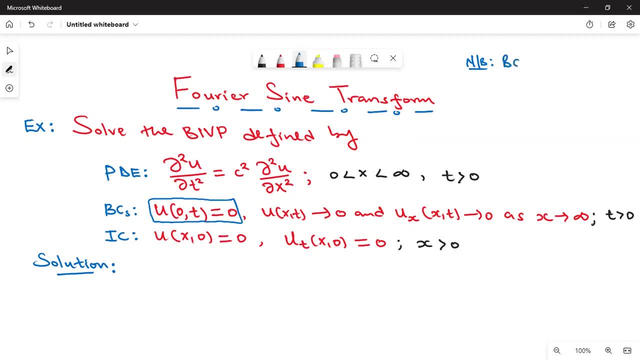 You look at boundary conditions at the lower end. The lower end- for this case it is at x- is equal to zero. So if you are told u over zero t, if this is given, then it means you use the Fourier sine transform. 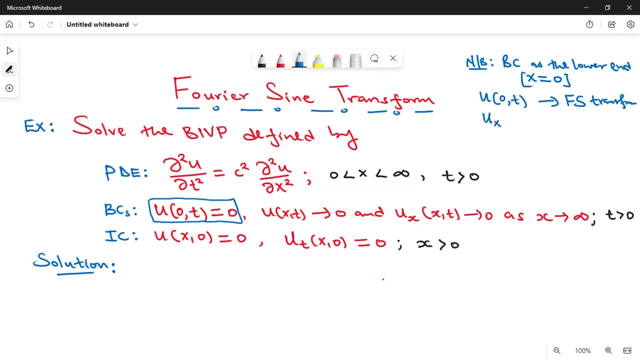 But if you are given u subscript, x at x is equal to zero t. Now look at: if you are given this boundary condition, then you use the Fourier cosine transform. So that is what will guide you between choosing between the two transforms. Now for our question. look at the boundary condition that you are given at the lower end. 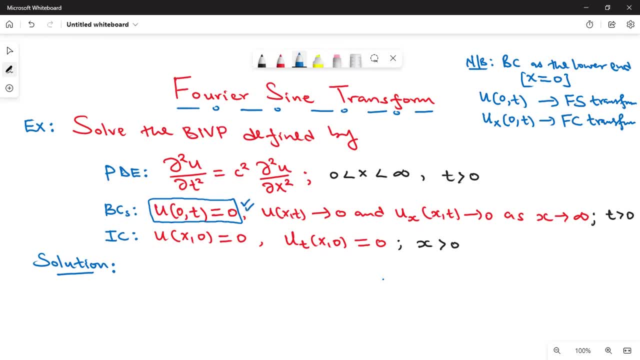 It is simply u of x, u of zero t, So I'm going to go for the Fourier sine transform, even if you are not told which one to use, That is, this is what will guide you on which transform to use Now, having explained this one, 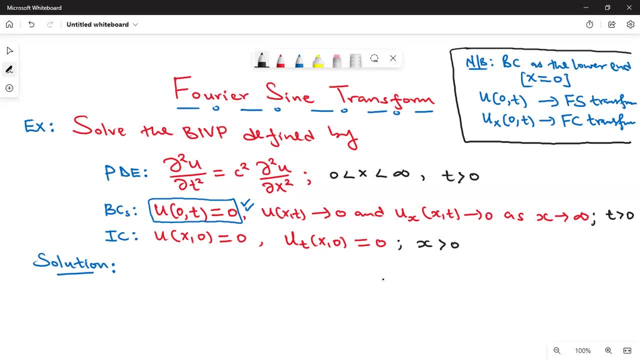 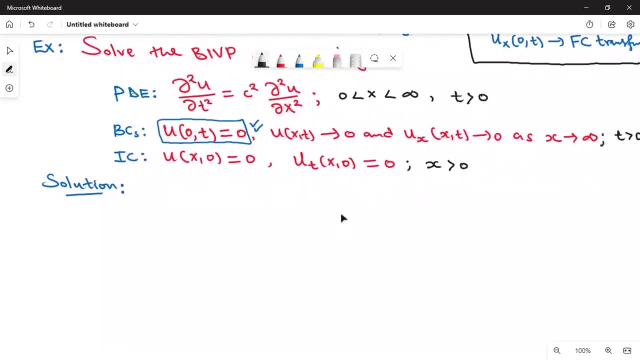 let's now go back to our question and solve it. Of course, the steps are as usual. You need to find, First of all we are going to say let let f subscript s denote the Fourier sine transform operator. It's operating in the variable. 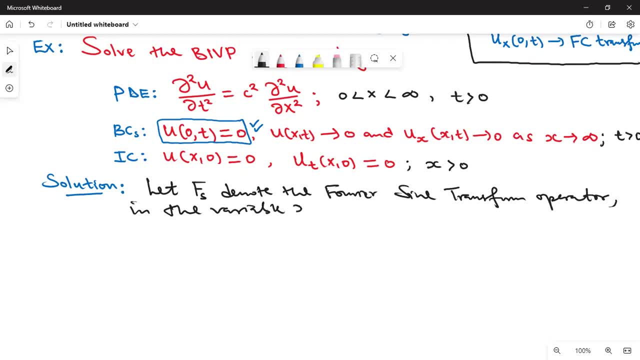 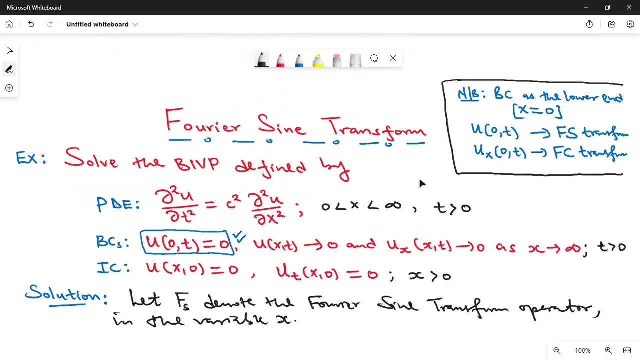 in the variable x. Now somebody might ask: what is the difference between Fourier sine, Fourier cosine transform and the Fourier transform, the complete Fourier transform? The difference here is that in Fourier sine and cosine transform our domain is semi-infinite. 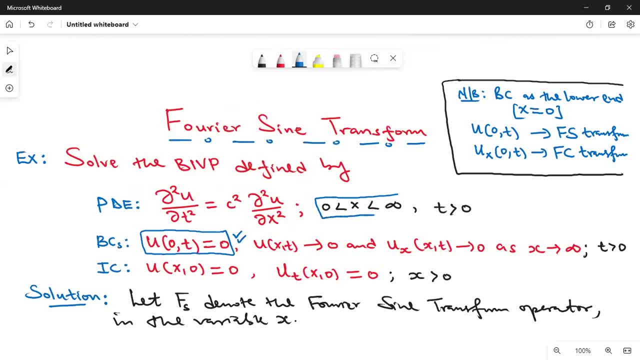 When you have a semi-infinite domain, just like this one, from zero to positive infinity, then you need to use either Fourier sine or Fourier cosine transform, And I've told you the choice. what will guide you on which transform to use? So, and when you have a complete domain from negative infinity, 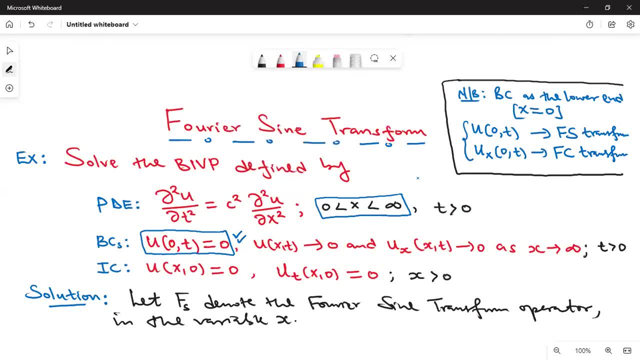 to positive infinity. in that case you cannot use Fourier sine or Fourier cosine transform. There you are going to use the complete Fourier transform, the usual Fourier transform, where you need to integrate from negative infinity to positive infinity. So you need to take note. 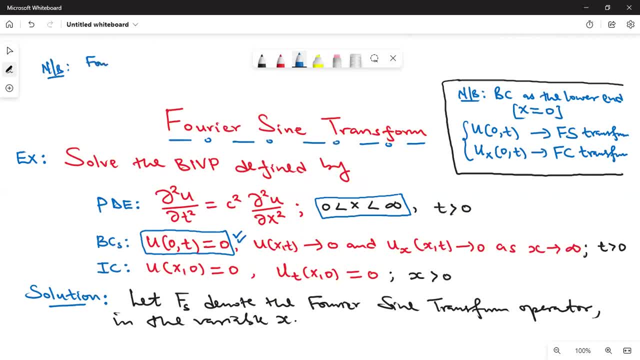 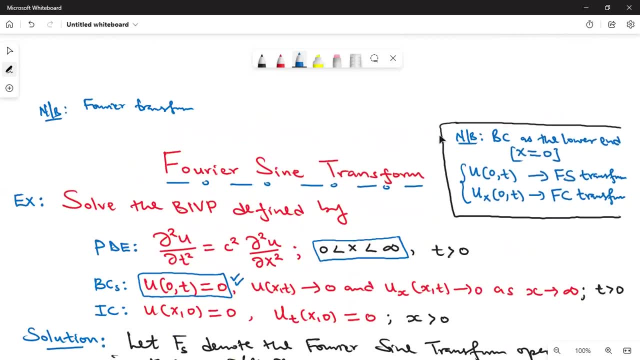 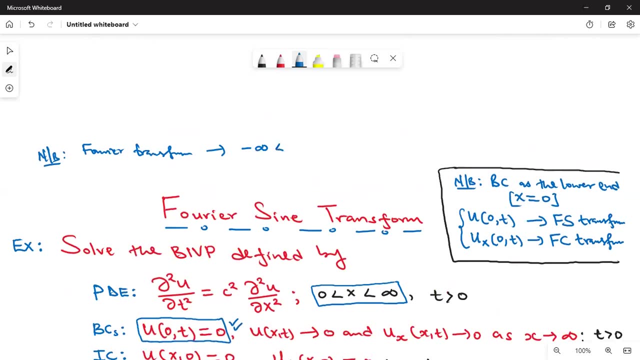 that when we talk of Fourier transform, Fourier transform, the domain extends from negative infinity, is from negative infinity, less than x, less than positive infinity. When you have such kind of a domain, you use Fourier, the complete, Fourier transform. We'll have written here: complete or complex. 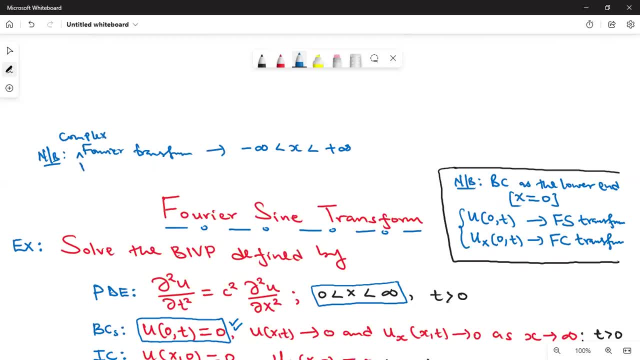 Fourier transform. But when we talk of Fourier sine transform or Fourier cosine transform, the domain is semi-infinite, is from zero, less than x, less than positive infinity. So this one is semi-infinite, This one is infinite. So when you have an infinite domain, 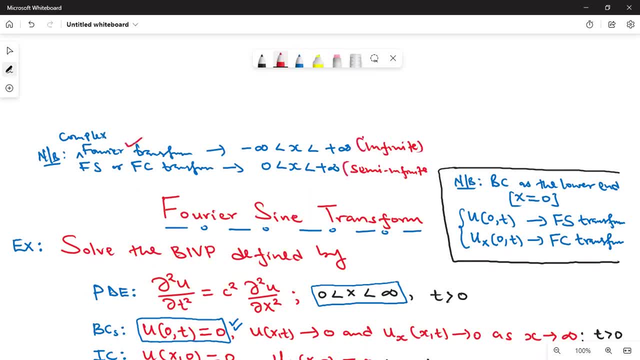 use the complex Fourier transform When you have a semi-infinite domain, use either Fourier cosine transform, this Fourier sine transform or Fourier cosine transform. So that's the difference between those three transforms And the difference between the Fourier sine transform and the Fourier cosine transform. 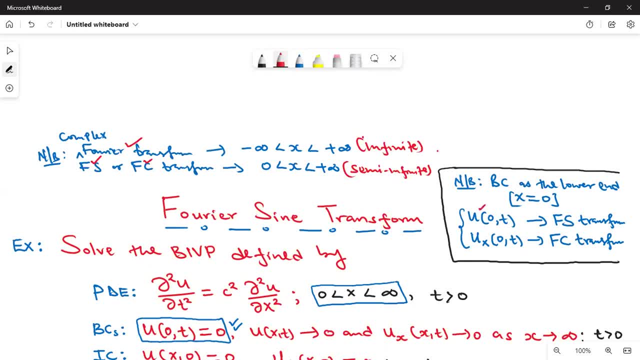 is you look at the boundary condition at the lower end. When you see the solution at the lower end as given, then use Fourier sine transform. But if the velocity at the lower end is given, velocity means we are differentiating. now then you use the Fourier cosine transform. 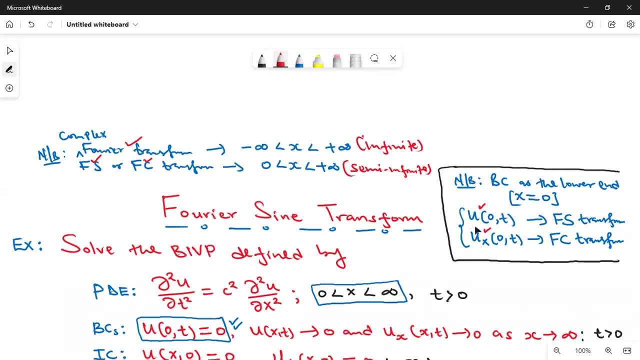 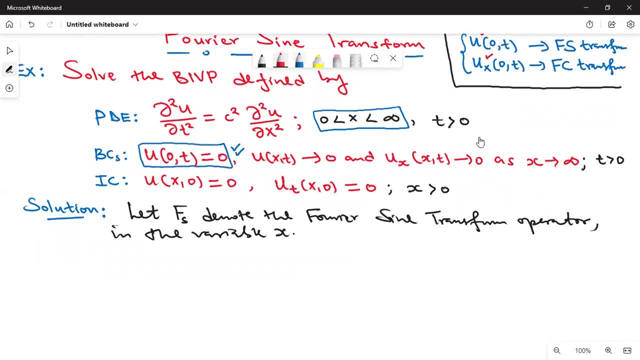 So I haven't explained those critical information. Let us now go back to our question and solve it. So here we have F, subscript S as our operator. That is the Fourier sine transform operator. It will operate on the variable x. So now the first step. 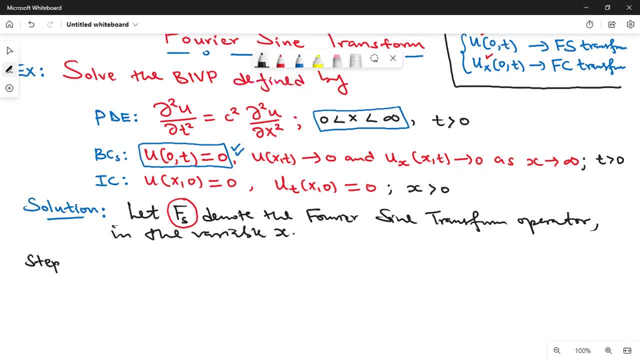 we will write here step one: What do we do? We operate with F subscript S on both sides of the PDE. So we operate with F subscript S on both sides of the PDE. So we operate with F subscript S on both sides of the PDE. 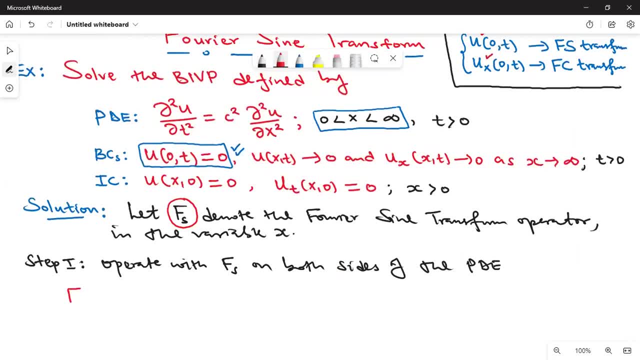 So that will give us the Fourier sine transform of second derivative of u with respect to t. twice is equals to Fourier sine transform of c squared second derivative of u with respect to x twice. That is just a constant which can be factored out. 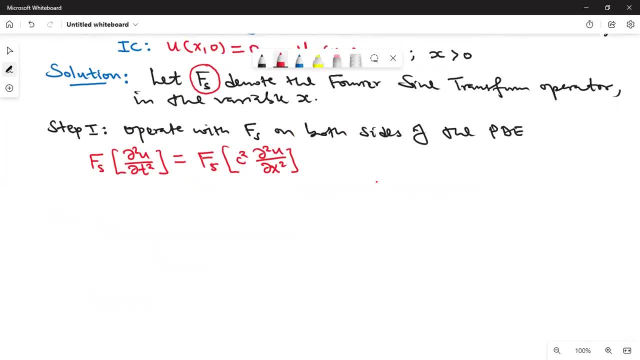 So when you take the transform, this is what we need to get. On the left-hand side, that will now be ODE, d squared, dt squared of the Fourier sine transform of u, of x, t. That's how it will be transformed. 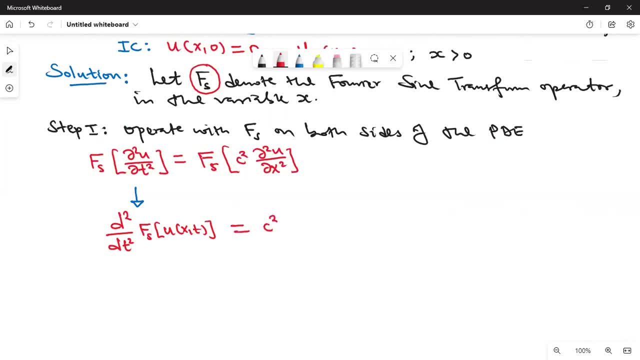 On the right-hand side I will have c squared times, the Fourier transform of second derivative of u with respect to x, t And that Fourier transform. of course we are not going to derive it because I expect that you know how to derive that Fourier transform. 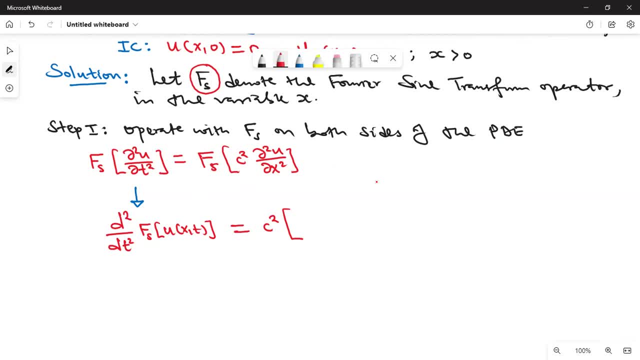 based on the given boundary condition. So this is what you are going to get as the Fourier transform of the second derivative of u with respect to x twice. It will give you omega times: u x zero, no, no, no, u zero x. 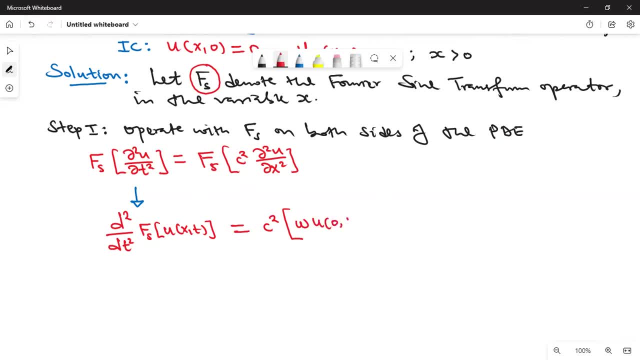 u zero t. I mean u zero t, then minus omega, squared times, the Fourier sine transform of u of x t. That's what you need to get. Somebody might be wondering why we are getting this form. This is the definition of the Fourier sine transform. 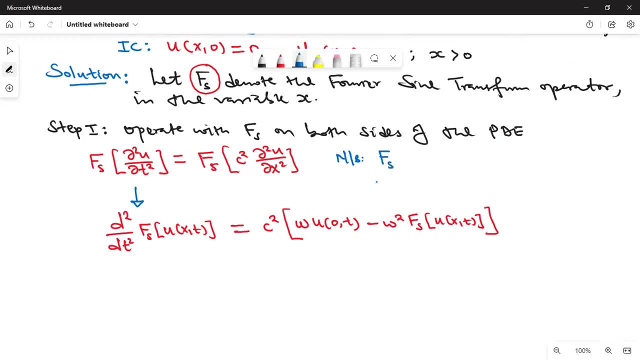 that the Fourier sine transform of any function, let's call it u of x, t- is equal to the integral from zero to infinity. Now here we will have sine omega x times u of x, t, dx. So that's how we define the Fourier transform. 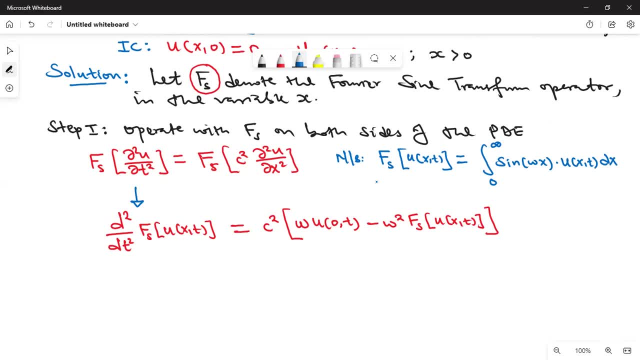 of any given the Fourier sine transform. I mean of any given function. So when you use that, you're going to get what we have found here. Of course you're going to use integration by parts, but I believe you already know how to derive. 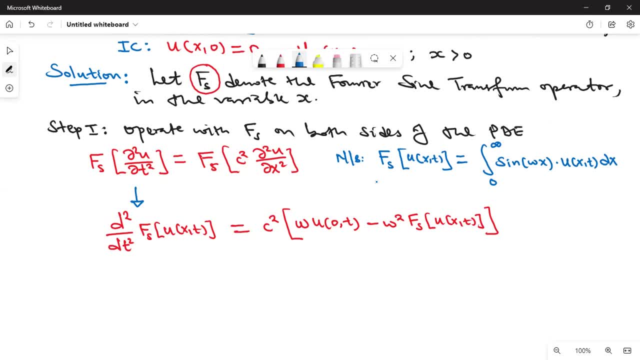 such kind of a transform. So, having known that one, let's now apply the boundary condition we are given. So the second step, step two: you now apply the boundary condition at the lower end. The lower end, that is, when x is zero. 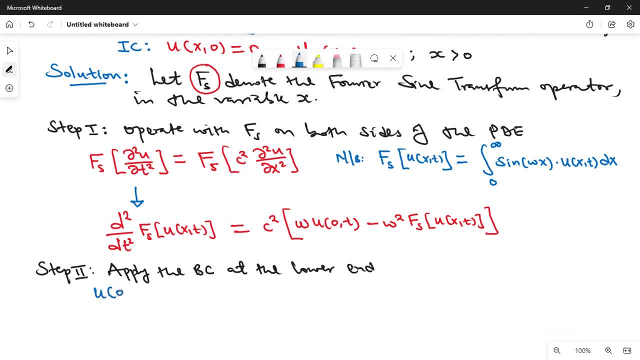 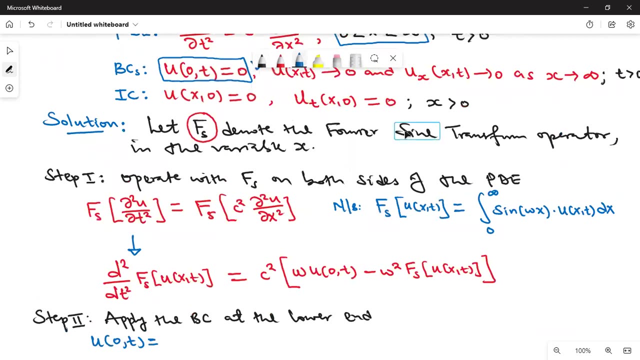 So we are given that u of zero, t is equal to, that is supposed to be equal to zero. So what do we remain with? Was it zero or one? Just a minute, I check The boundary condition at the lower end for this equation. 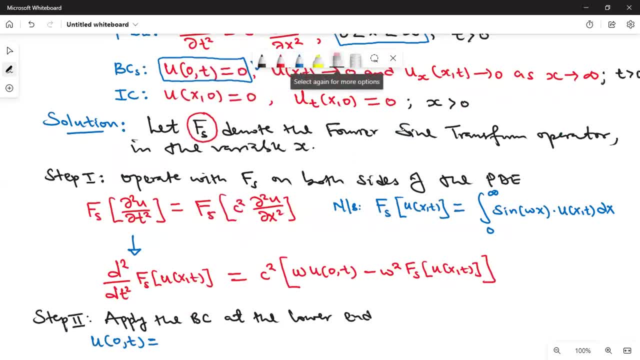 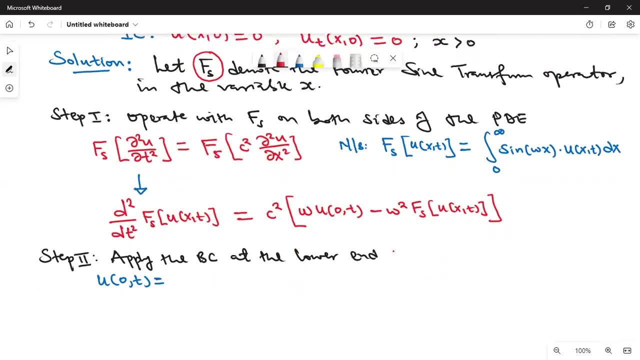 this problem. it was one. I've written zero by mistake. This condition is given as one. Let's have it as one. So let's apply that Where there is u of zero t, you need to write one. That means this value here. 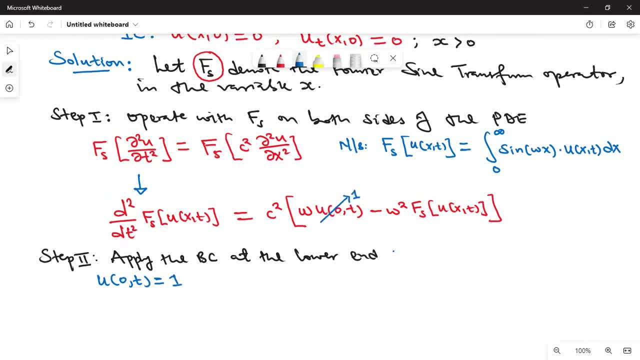 is one. So one times omega, that will just be omega. So what will be our equation? So therefore, the ODE will now be d squared d, t squared of the Fourier sine transform of u of x, t is equal to c squared. 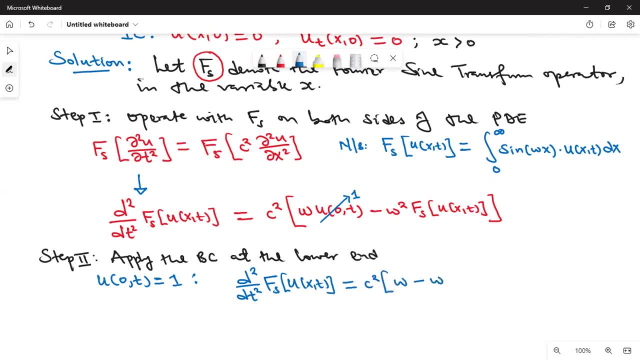 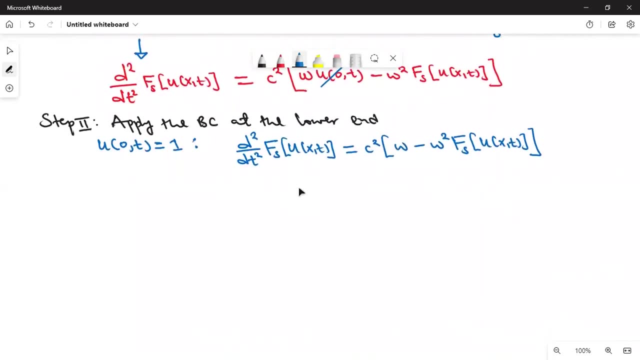 into omega minus omega squared, Fourier sine transform of u, of x, t. That's what we have. You can also rearrange it. You can also rearrange this so that you get, you can write ODE, d squared, d, t squared of the Fourier sine transform. 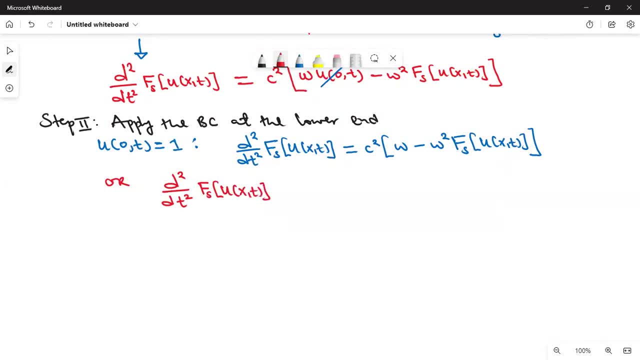 of u, of x, t. Then now I want to take this to the left hand side, So it will become plus c squared, omega squared times the Fourier sine transform of u of x, t. And now, on the right hand side, we now have c squared. 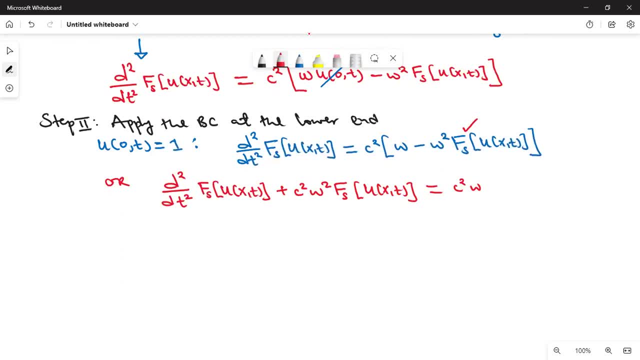 omega. So I can use d operator. So you can say: let let d be derivative with respect to t. So this will imply that if I want d squared, there will now be the second derivative with respect to t twice. Remember, this is an ODE. 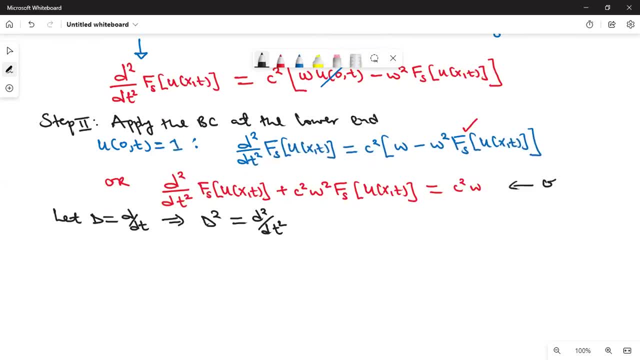 So, therefore, this one is an ODE of second order with a constant coefficient. So our ODE will now look like this: In terms of the d operator, it will now be d squared plus c squared, omega squared times the Fourier sine transform. 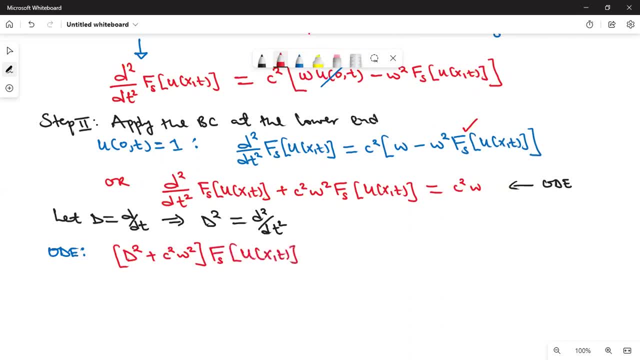 of u of x t. Of course no time. but it should operate because an operator is operating on a function So that d squared plus c squared, omega squared, is operating on the Fourier transform, Fourier sine transform of u of x t. 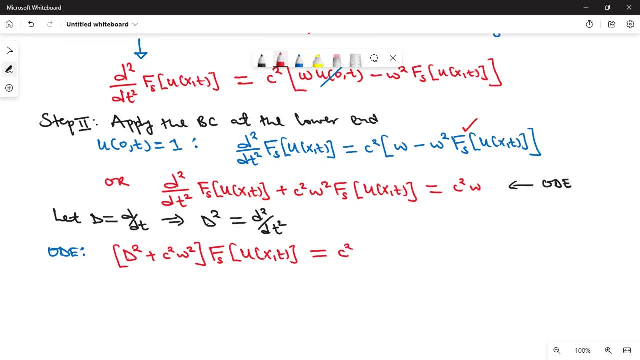 to give us c squared omega. This equation is homogeneous. I said it is ODE second order, non-homogeneous- non-homogeneous with constant coefficients. It is also linear, Linear, second order ODE, non-homogeneous. 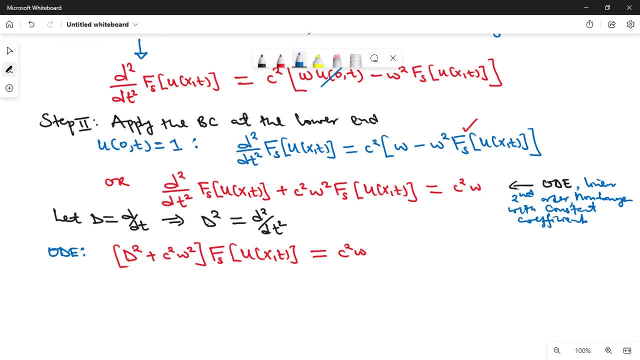 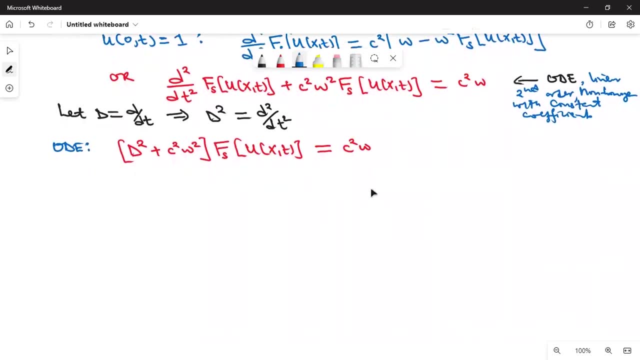 with constant coefficients. So how do we solve this kind of equation? There are two types of solutions. The first one is the complementary function. Another one is the particular integral. So let's start by finding the complementary function. Complementary function: this means I'm going to solve. 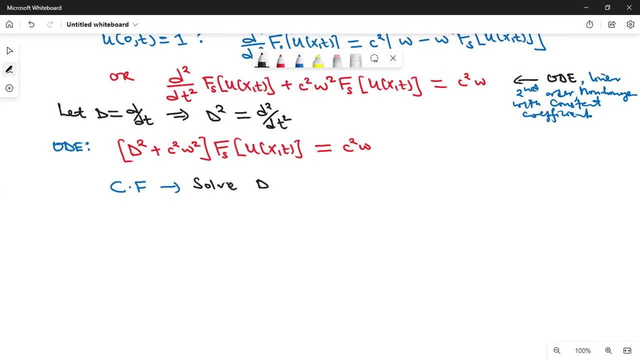 solve the homogeneous part, that is d squared, plus c squared, omega squared, operating on the Fourier sine transform. Now I'm going to call this function u c of x, t u c, to mean: okay, let me now try, because that will confuse us a lot. 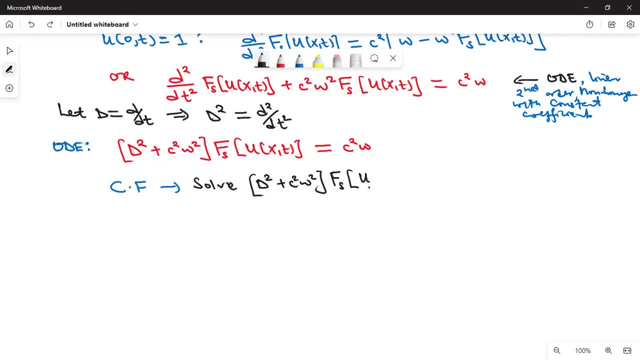 u, c to mean, let me write u of x, t is equals to zero. So what is the auxiliary equation, Auxiliary equation that is, d squared plus c squared, omega squared is equals to zero. So that the roots here 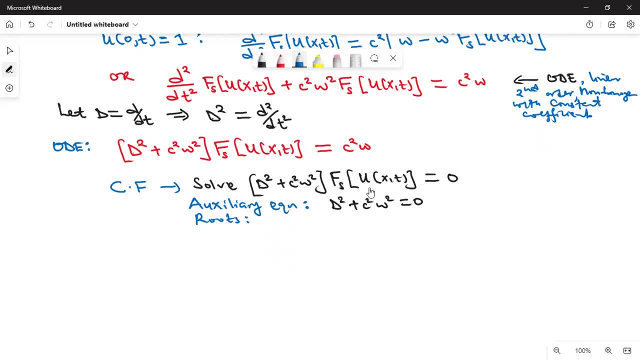 we have two roots, that is, d one and two. d one and two is the square root of negative c squared, omega squared. And you know, square root of a negative number is a complex number. So this would be plus or minus i at a times c omega. 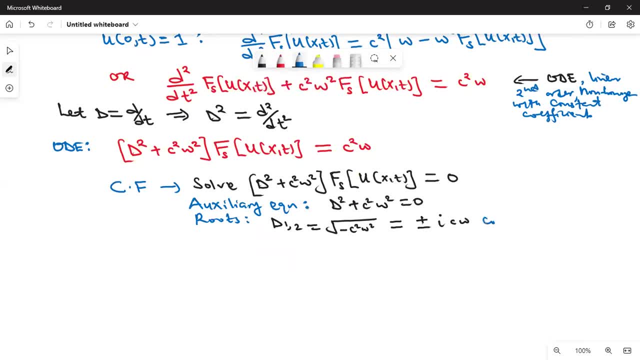 So these roots are complex conjugates, Complex conjugates, Complex conjugate roots. So therefore, your solution, therefore our complementary function is equals. to call it c one cos c, omega. This is a t cos c, omega, t plus c two. 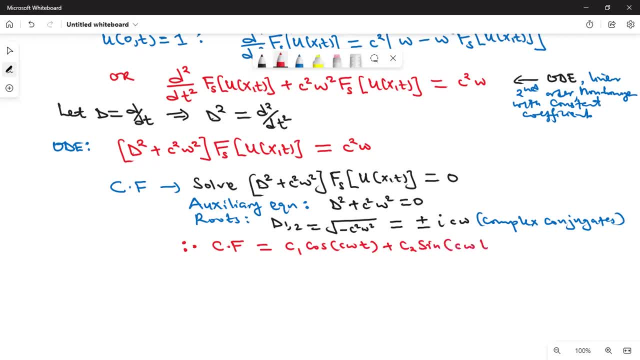 sine c, omega t, Where c one and c two are arbitrary constants. So that is complementary function. Let's find the particular integral, Particular integral. You need to make that Fourier sign, transform the subject Of the formula. Remember, this is what you are solving. 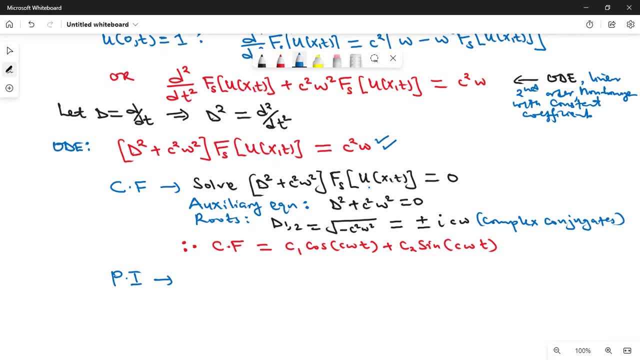 This one, So particular integral it is equals to one over d squared plus c squared omega squared Operating on c squared omega. So that is what we have. So how do we, how do we find it? That's the question. You see, c squared omega is a constant. 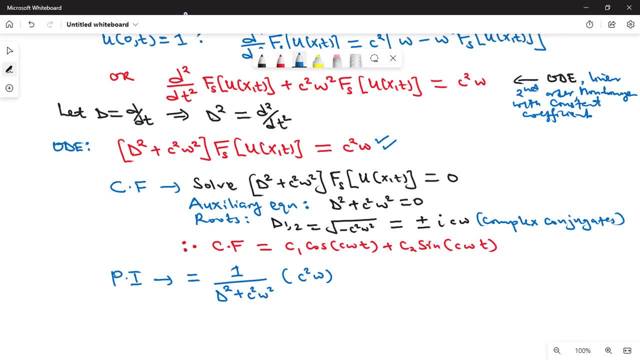 It's a polynomial of degree zero. It's a polynomial of degree zero. Polynomial of degree zero. It is a constant. So then it means you are going to drop the, the powers of d, Or those terms of d with higher powers than the degree of the polynomial. 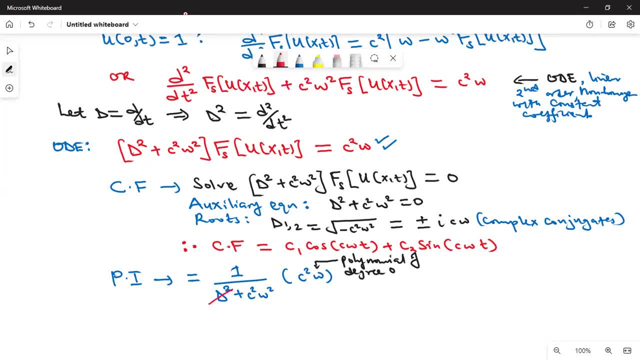 I'm going to drop d squared, because d squared two is greater than zero, So you drop it, So that what you remain with is one over c squared omega squared, then times c squared omega, And so this will give you- because I can see that c squared will cancel. 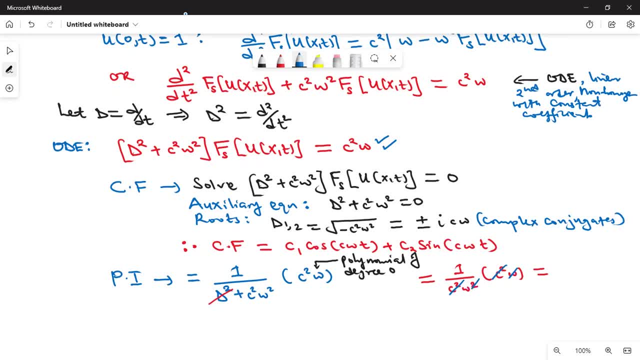 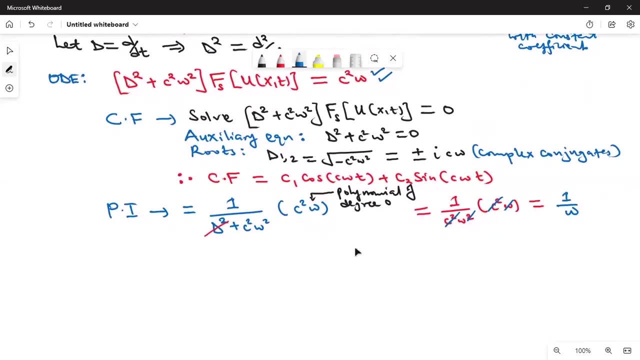 And even the omega will cancel with one of the omegas. So we still we just have one over omega as our particular integral. So therefore our general solution is the sum of those two solutions: Complementary function and particular integral. So the general solution. 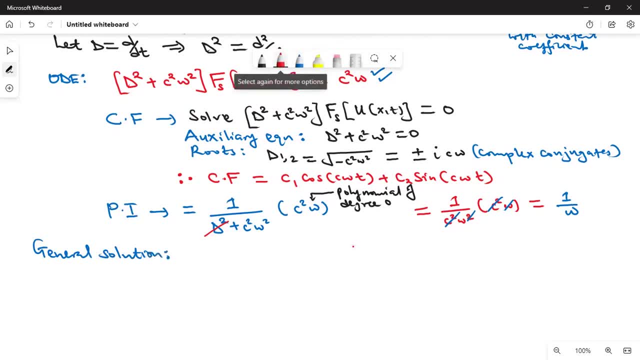 is given by the Fourier sine transform of. let me write this general solution is simply equal to complementary function plus the particular integral, Or what we write to: the Fourier sine transform of u, of x, t Is equal to the other one. we got c, one cosine. 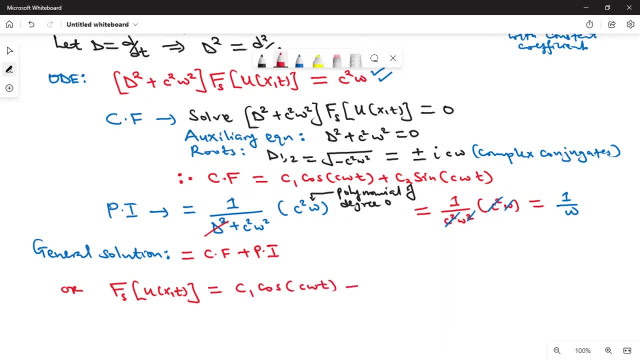 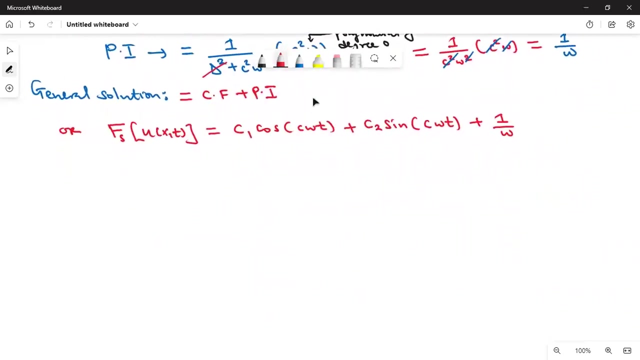 of c omega t plus c, two sine of c omega t plus one over omega. That's what we have Now. we have the initial conditions that we need to apply. So that's the third step. You can write step three: Apply the initial conditions. 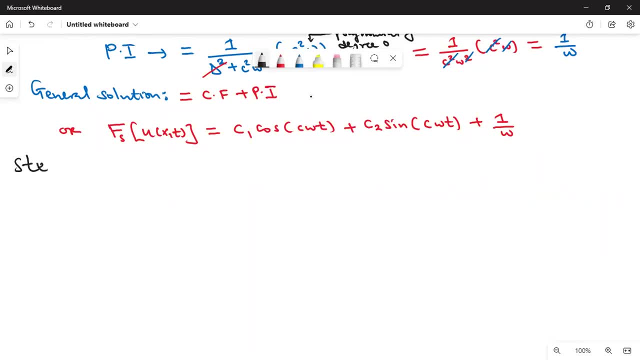 So you write step three Here we now apply the initial conditions. So what is the first one? We are told: u x zero is equal to zero. So the first condition is that u of x zero is equal to zero. So because, look at our 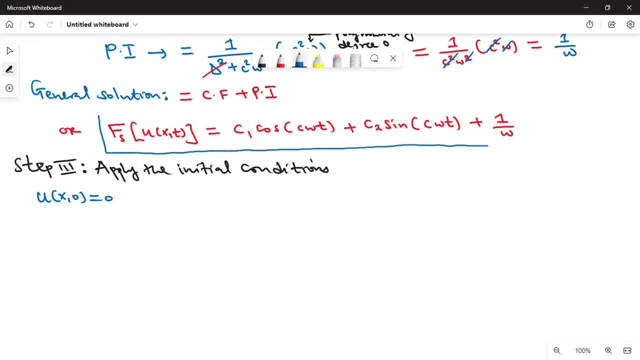 general solution is: it is in terms of the Fourier sine transform. So before I apply the initial condition- u x zero is equal to zero- I must also know the transform of that initial condition. So this means that Fourier transform, Fourier sine transform of u of x zero. 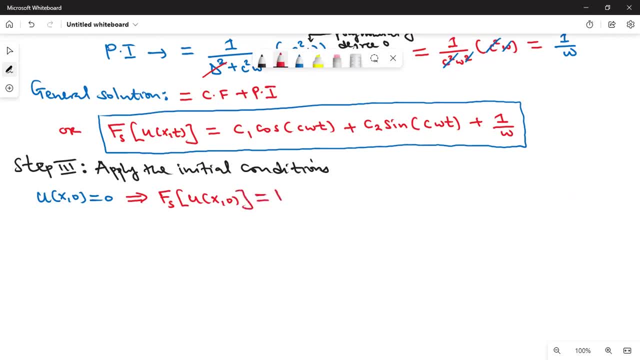 will also be equal to the Fourier sine transform of zero, And that will give you u of x, zero. So that means on the left hand side I'll write zero And when I put, t is equal to zero on the right hand side. So therefore, 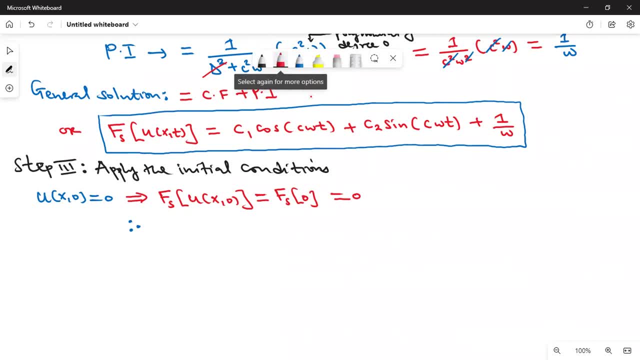 you can just say that therefore, zero on the left hand side we are substituting here, We are putting t- is equals to zero in that equation to get the solution to be zero. So zero is equals to, and remember, cosine of zero is one and sine of zero is zero. 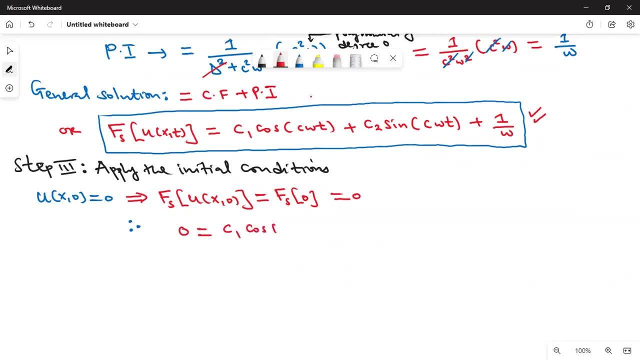 So this is the same as c one. cosine of zero plus c two. sine of zero plus one over omega. So just like I've said that sine of zero is zero, So this term will vanish and cosine of zero here is one. So we only have c two times one. 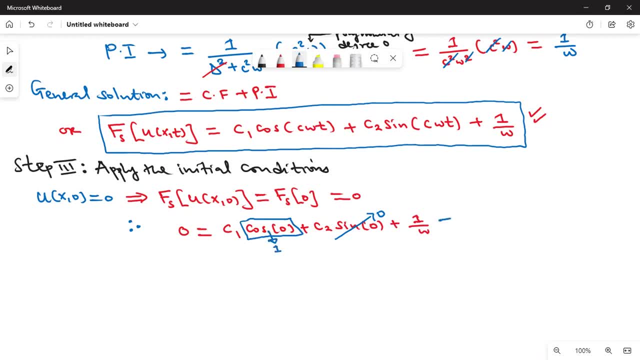 This is one, So this implies that zero is equals to c one. the c two is not there because that is times zero. So then plus one over omega, So or c one is equal to negative one over omega, So that's the value of c one. 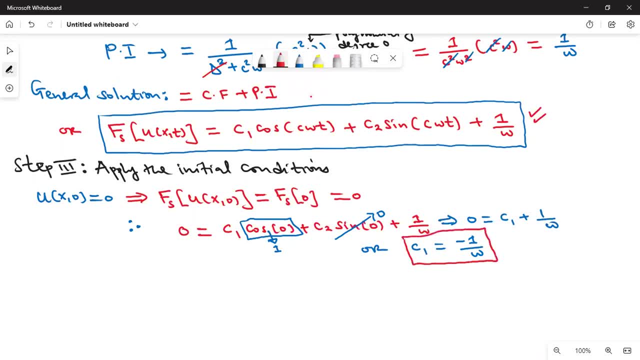 Negative one over omega, So let's replace it back. So hence, you can just say hence. hence, if I replace c one by negative one over omega, what are we going to get? We are going to get: Fourier sine transform of u of x, t is equals to: 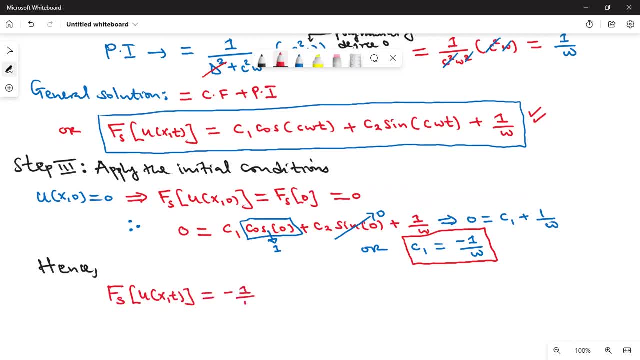 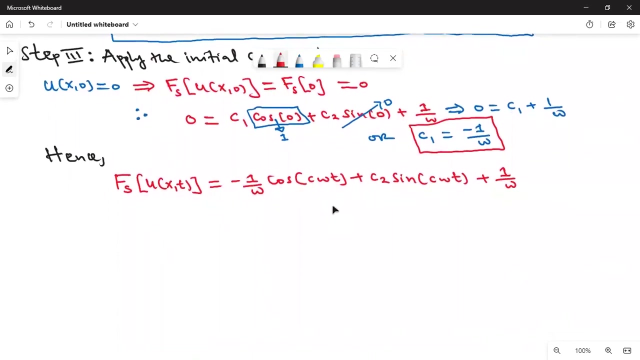 negative, one over omega. Then here we have cosine of c, omega, t plus I don't know c. two then sine c, omega, t plus one over omega. There's another initial condition to be applied: The derivative of u with respect to t. So let me differentiate this. 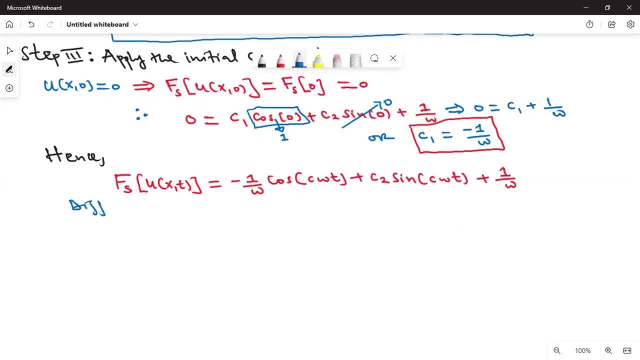 So we are going to differentiate, differentiate with respect to t on both sides. So what are we going to get when we differentiate? We are going to get Fourier sine transform of u, subscript t of x, t. I've differentiated it with respect to t. 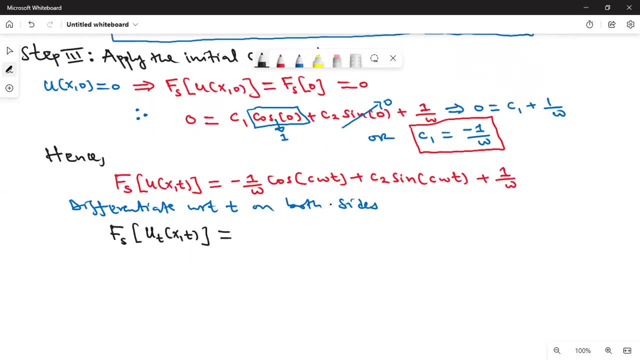 What about the right hand side? Derivative, of course, is negative sine, So this should be equal to negative. of course negative sine will come with the other negative, So that what we'll have is just positive c omega over omega, So positive c omega. 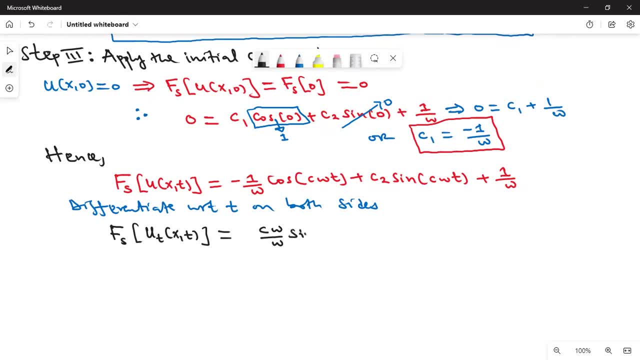 over omega, then sine c, omega t. The other one: differentiate sine you get cosine, So we have c two times c, omega cos, cos c, omega t. And the other one is a constant which when you differentiate you get zero, So which I don't even need to write. 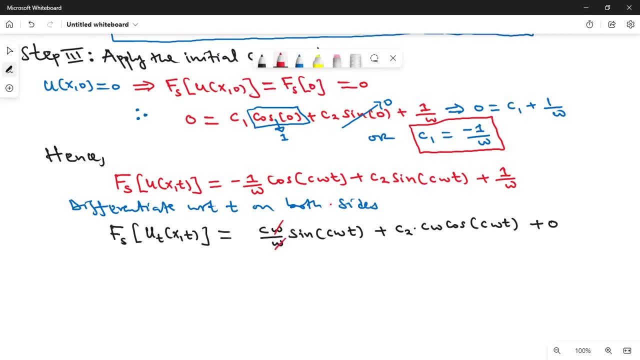 and you see, here I can see omega will come with this other omega. So you can write this as c sine times c, omega t plus c two times c, omega, cos c, omega t. That's what we have On the left hand side. you can just write. 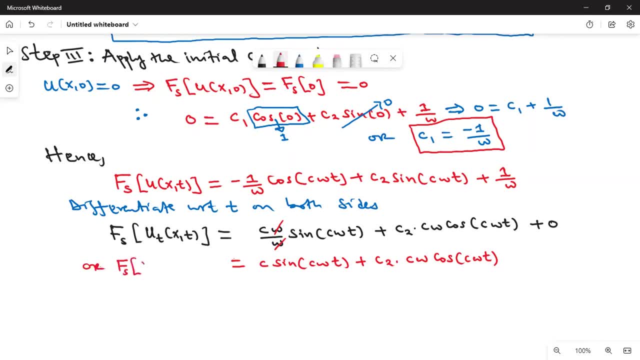 Fourier sine transform of u sub fifth t of x. t is equals to that. So now we need to apply this condition: Apply u sub fifth t of x. zero is equals to zero. So from here, what does it mean? That if I take the transform, 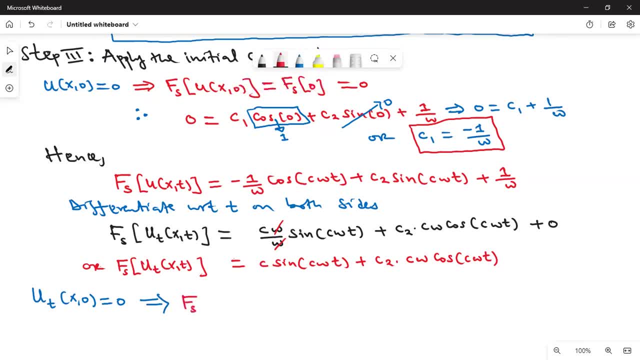 on both sides. I'm going to get Fourier sine transform of u sub fifth t of x. zero should be equal to the Fourier sine transform of zero, which is equals to zero. So that means that in this equation, in this equation, the one that I am bracketing- 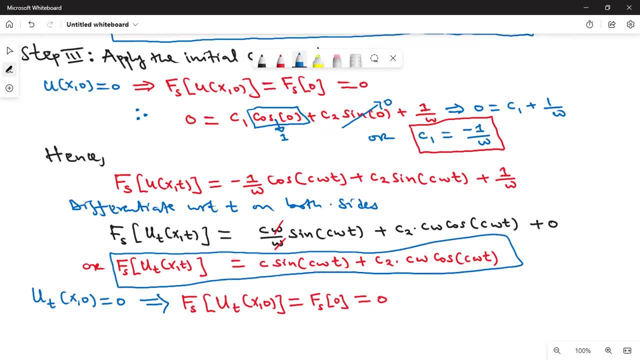 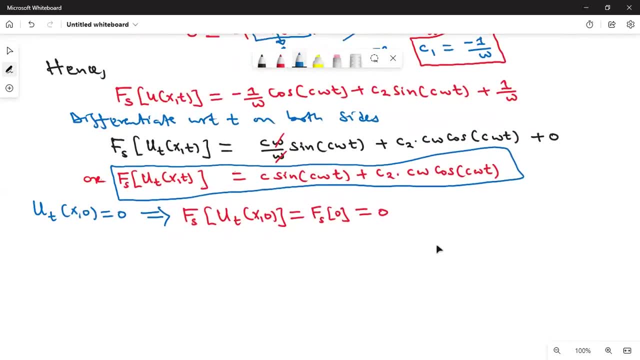 if I substitute, t is equals to zero. I need to get that transform to be zero on the left hand side. So therefore, upon substitution, we are going to get. you can just say, therefore, zero is equals to c times sine zero, because t is zero, c times sine zero. 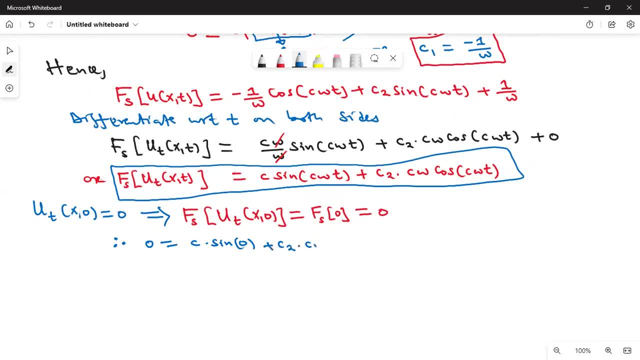 plus c, two times c, omega times cosine of zero. and you know sine zero is zero. so I don't expect this. this would be zero and cosine of zero is one, so this is one. so what do we have? is that zero on the left hand side is equals to: 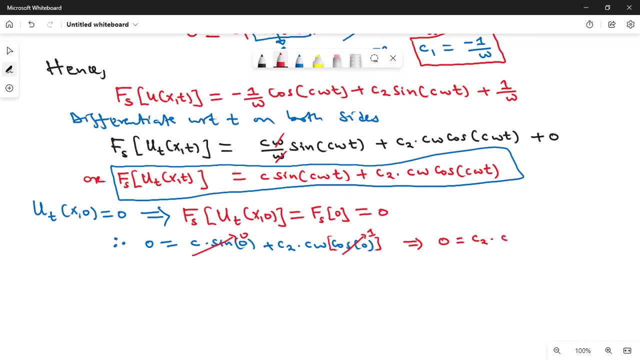 c two times c- omega. When I divide by c- omega, I am going to get: c two is equals to zero. because you see, c is not equal to zero, omega is also not equal to zero, so it is c two that is equals to zero. So remember, c is not equal to zero. 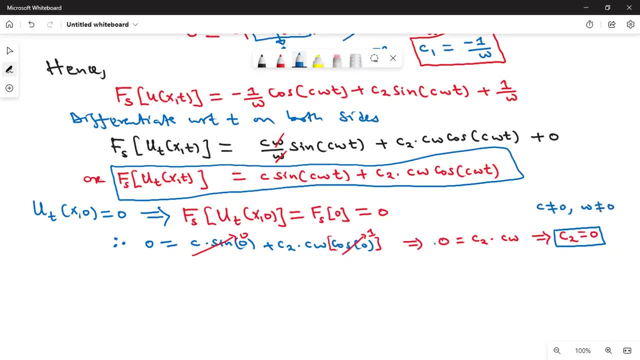 omega is not equal to zero, So c two must be equal to zero. So therefore we come back and replace it here. you can just now see that. hence the Fourier sine transform of u, of x, t should now be equal to. I have replaced c two to be zero. 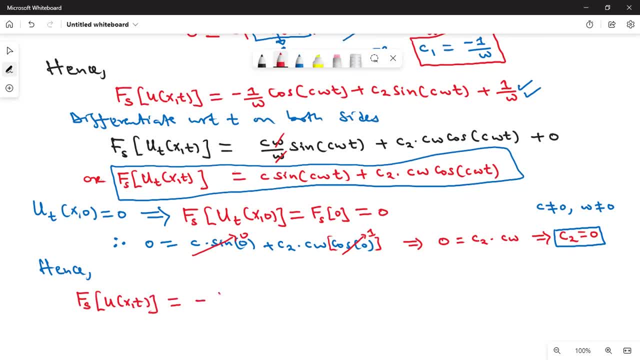 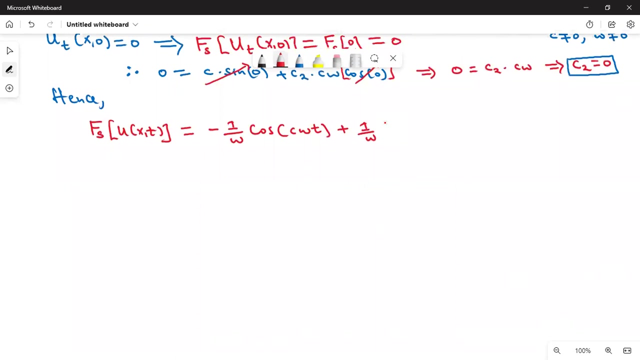 so I am just going to get negative one over omega. Okay, So we have cosine of c, omega, t. the other one is zero. so we will have plus one over omega. and how else can you write this? you see, one over omega is common, but this can be written as: 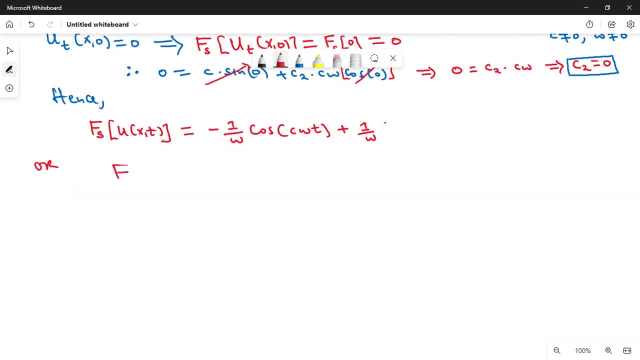 you can just say: or the Fourier sine transform of u of x, t is equal to one minus cosine of c, omega t, everything you divide by omega. So that is what you are getting and you can simplify this further. remember that one minus cross two theta. one plus two theta. 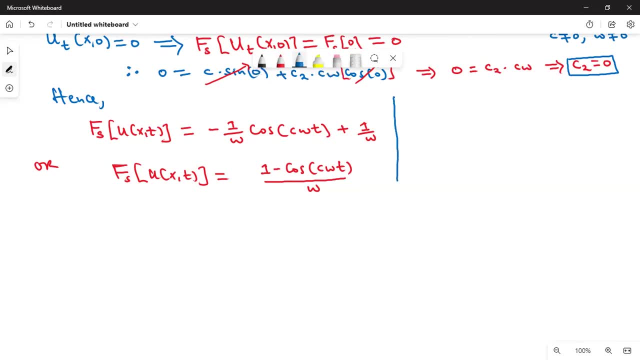 I want us to take note- take note here- that when we talk of sine squared theta, sine squared theta is usually equal to one over two into one minus cosine of two theta. there is a closing bracket before this one, so I need to close this, but I don't need to express. 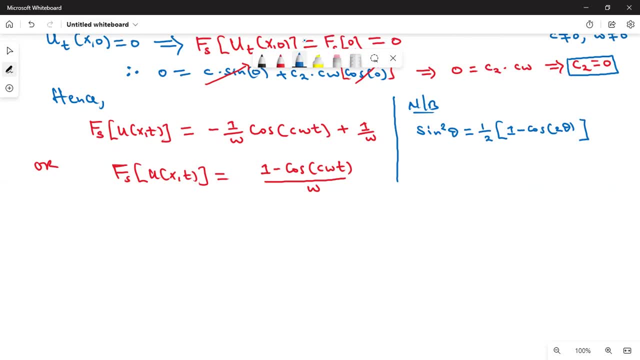 that in terms of sine squared, because it will make our work difficult when integrating, but I just wanted to bring to your attention that identity which you can use when there is a need. now, the last step, the last step, step four, is now operate with with F subscript S. 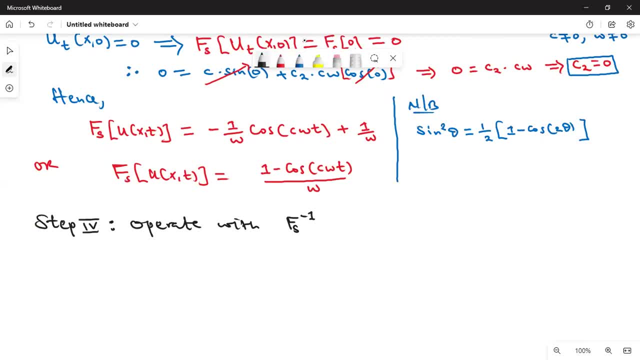 inverse. that means the inverse. Fourier sign: transform. you operate with it on both sides of this equation, the one that I have bracketed, this one we can call it star star. I hope you have somewhere. so operate with f s inverse on both sides of equation: star star. 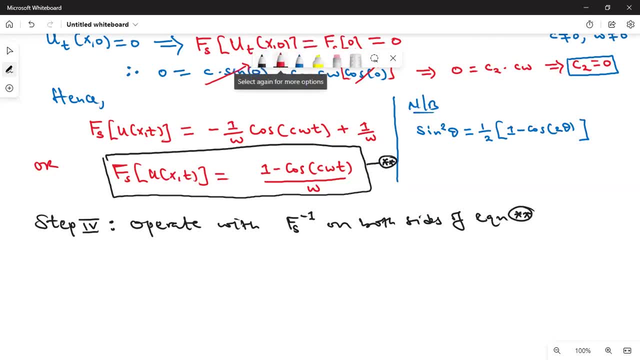 so when you operate on the left hand side, you are going to get u of x, d, remember f inverse and f, f. of course, f s inverse and f subscript s are inverses, and so when you operate on on them, you get the identity operator and identity operator operating on any function. 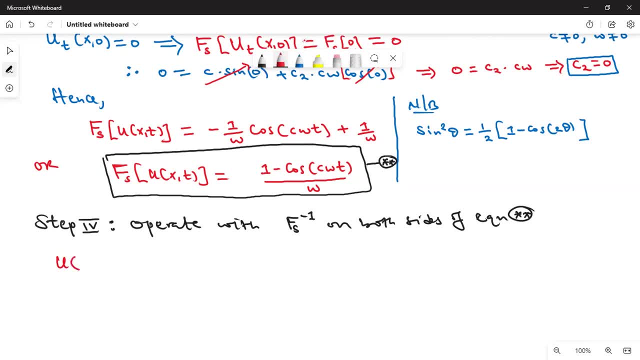 gives you the same same function. so on the left we'll have u of x, t is equals to. on the right we have f, f subscript s inverse square root of u of t, plus one minus cosine of c, omega, t, everything over omega. i want us to recall the definition of the inverse of Fourier, sine transform of any given function. 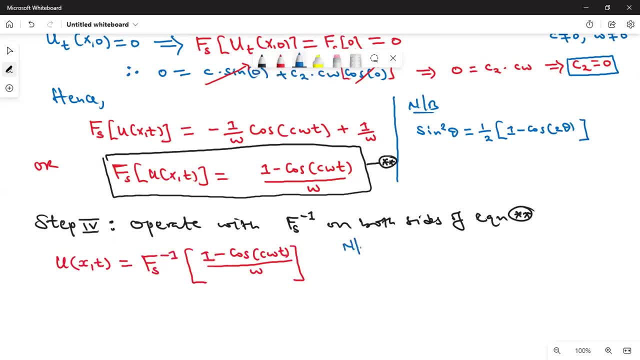 let's take note when we talk about of f subscript s inverse of any function of omega quality: u, capital of omega t. It is defined by 2 over pi times the integral from 0 to infinity of the function. you are getting its inverse, that is, u of omega t. 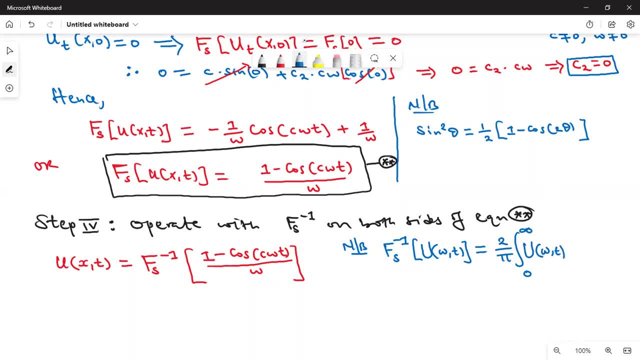 that's the function you are getting, its inverse times: sine omega x, d, omega. That is what we call the inverse Fourier sine transform. Inverse Fourier sine transform of the function u of omega t. Now we want to follow the same idea to now find the inverse. 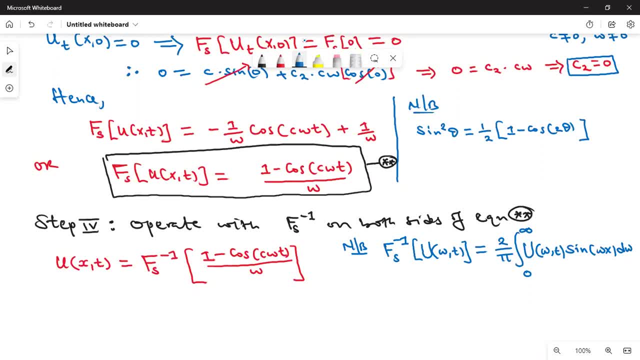 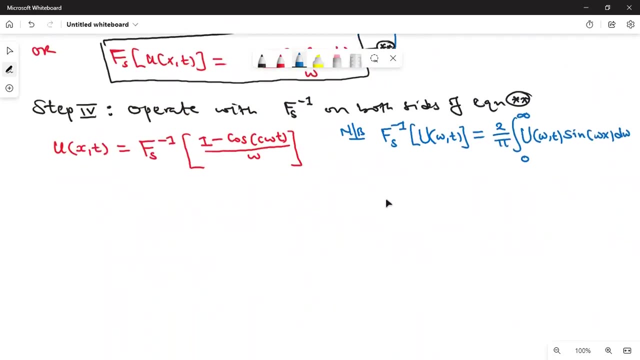 Fourier sine transform of what we have there and remember when you find the inverse, you will go back to a function of x and t- that's very important- where x extends from 0 to infinity. so therefore, this one can now be written as: this one you can now write as: 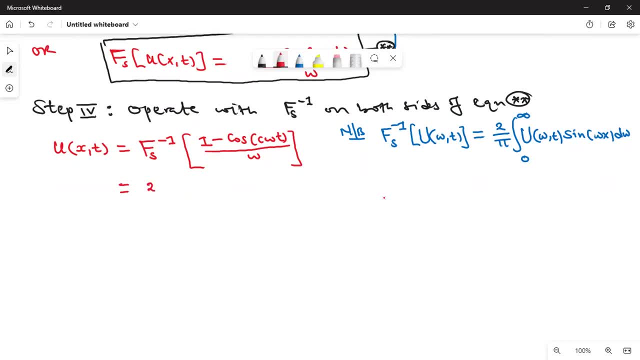 2 over pi, the integral from 0 to infinity of 1 minus cosine of c, omega t, and then you can write this as y of omega t over omega. this you multiply by sine, omega, x, d, omega, and if you know, you see, you can be able to work out this. 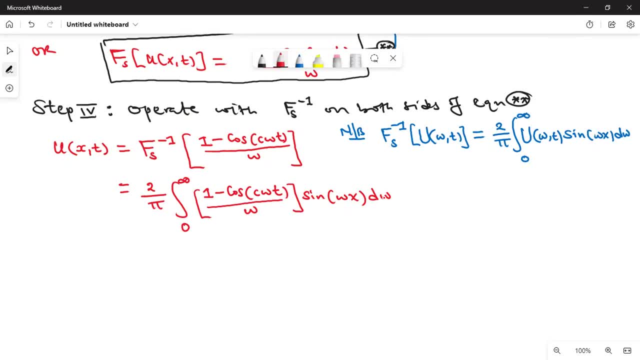 kind of integral, But you can as well leave your answer in this form, but you can let me know if you have any questions. if you have any questions, then I'd be happy to answer them. Thank you, this integral can be can be simplified, so what we have there is what we are calling the solution.